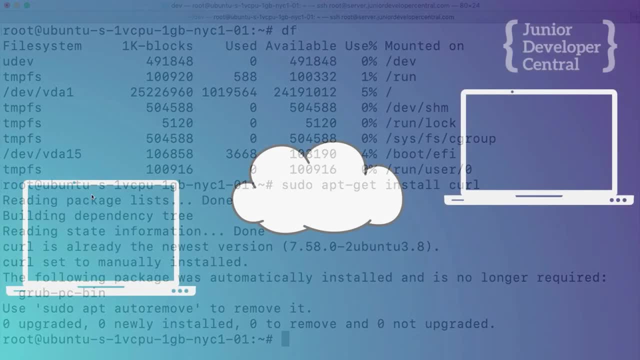 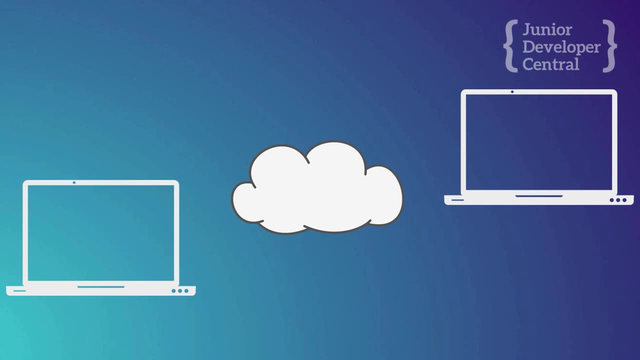 machine and run pretty much any command you need to. The problem with connecting to a remote machine over the internet is that your data will pass through many networks, some of which could be unsecured and have malicious programs or users listening for interesting requests. For example, if you were trying to run a command on a remote 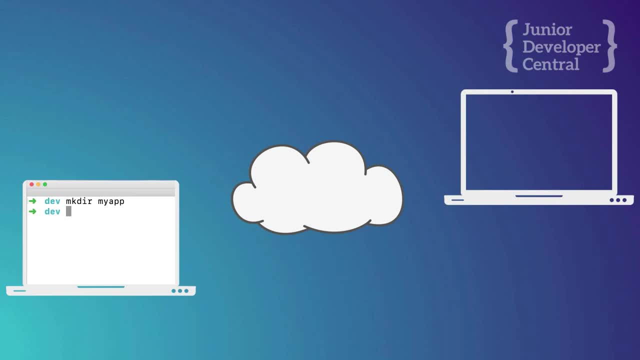 server from your local computer. over the internet, your transmission could be intercepted, viewed and possibly modified before it reached its intended target. SSH prevents this by creating a secure connection between the server and the internet connection between the two devices, where you can safely send requests to run commands on the remote. 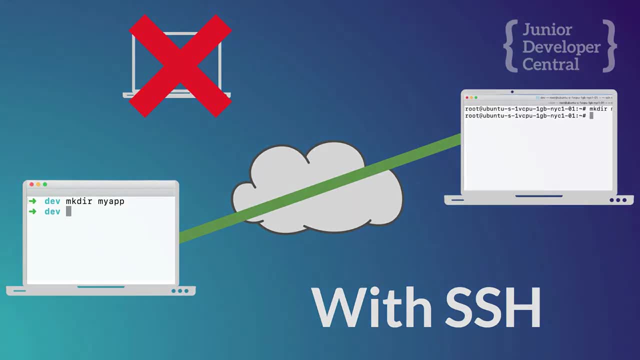 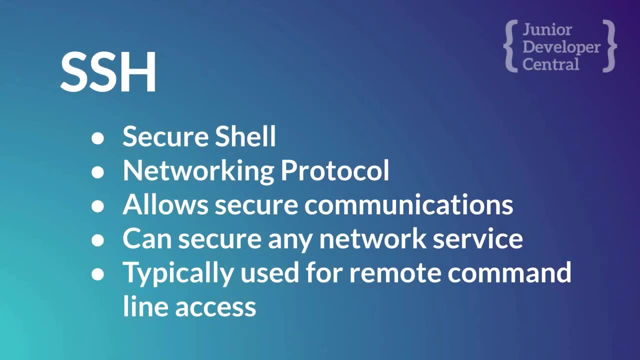 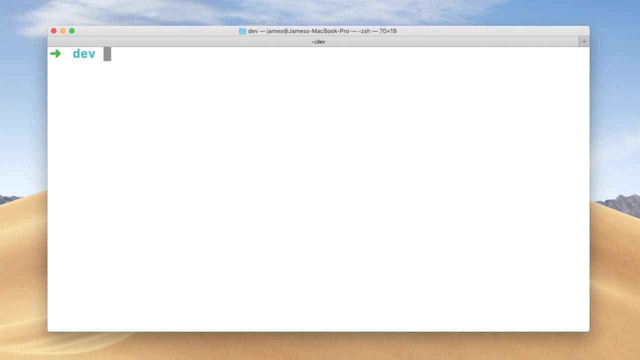 server. SSH can also be used to secure any type of network resource, for example HTTP or FTP, and we'll take a look at some examples at the end of this video. Generally, you would set up an SSH connection in the terminal or command prompt and you'll need to have both SSH server software. 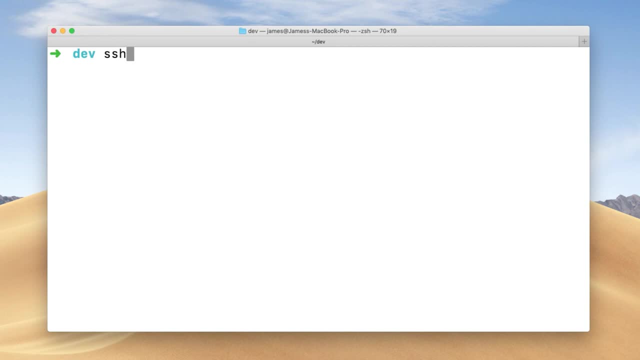 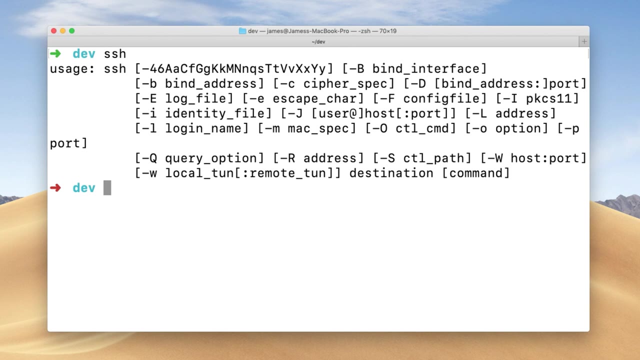 running on the remote machine and also an SSH client on your local machine to make a connection. This is something that's generally configured on new servers when they're set up. otherwise it'd be difficult to administer them, and Mac and Linux computers will have an SSH client installed. 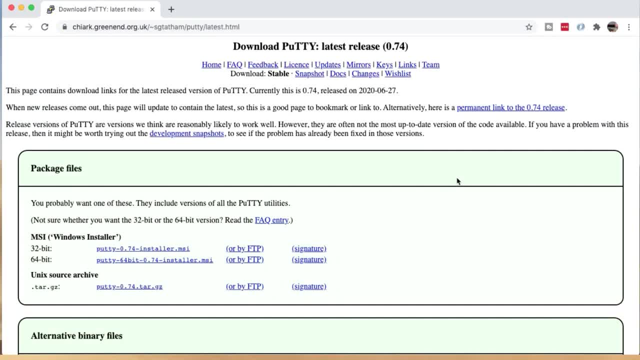 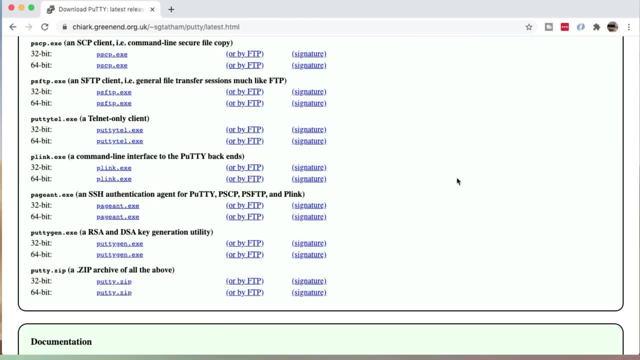 already For Windows users. either using a Unix-like command prompt like Git Bash or the Windows subsystem can provide command line access, or you can use the PuTTY client to manage connections. To make an SSH connection you need to know at least two things: The server host and the 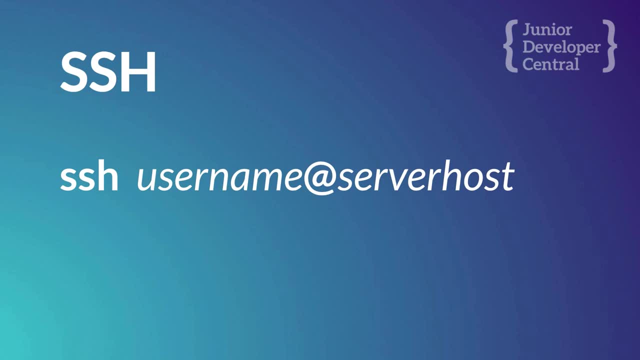 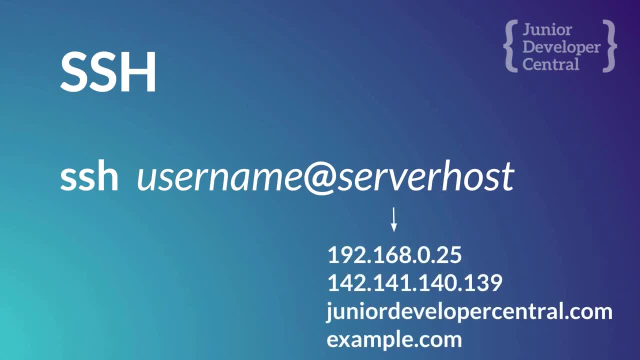 address or domain name. The username will be the user on the remote server that you're connecting to, not the user on your local computer. You'll also need some way of authenticating yourself to the remote server, which can either be a password or a key. We'll look at keys in a 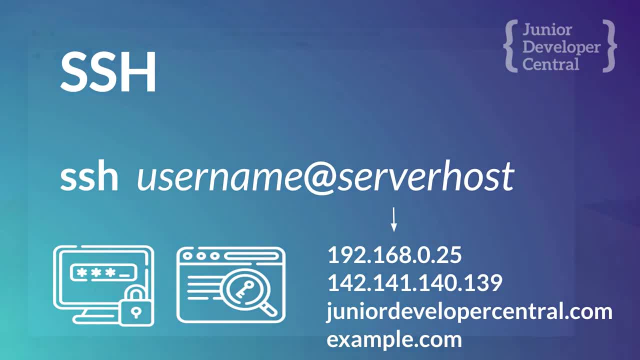 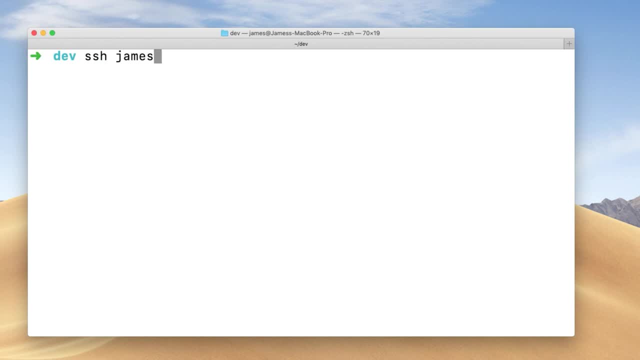 moment, but first let's make a connection to a remote server with a password. I'm going to connect to a remote server I have set up with DigitalOcean. First I'll type in SSH, James and the IP address is at 142.93.58.60, where James is my username on the remote server and the IP address. 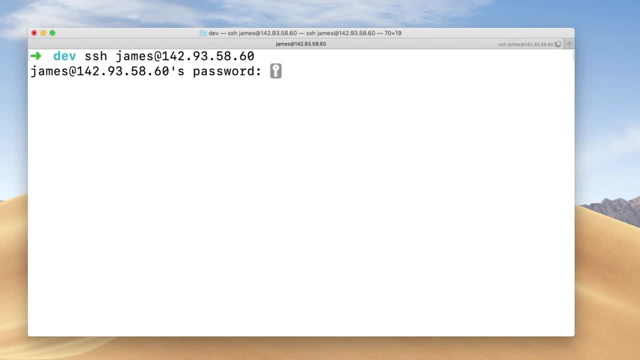 is the server host. I'll then be prompted for a password, which is hidden on the command line, so it needs to be typed in carefully. You might see a warning message asking you to accept the server's fingerprint, its identity, so type yes, if you trust the resource that you are trying to connect to. 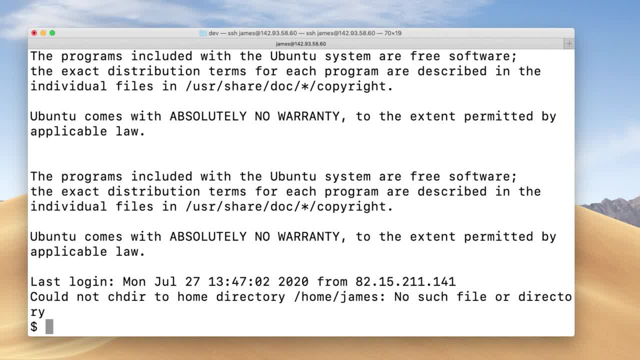 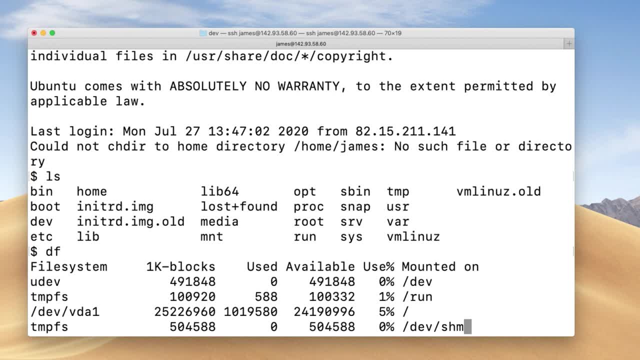 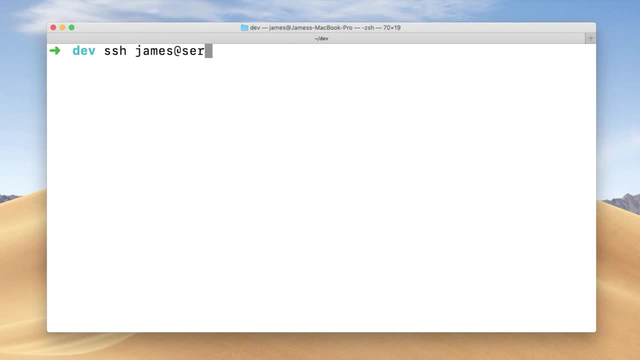 If the username and password are correct, you'll see the welcome message of the server and can happily execute any remote commands that might be needed. Let's try that again with a domain name instead. This time I'll type SSH James at serverjuniordevelopercentralcom. So now I'm using serverjuniordevelopercentralcom. 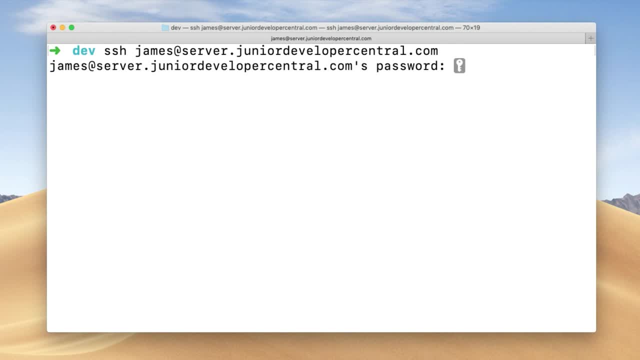 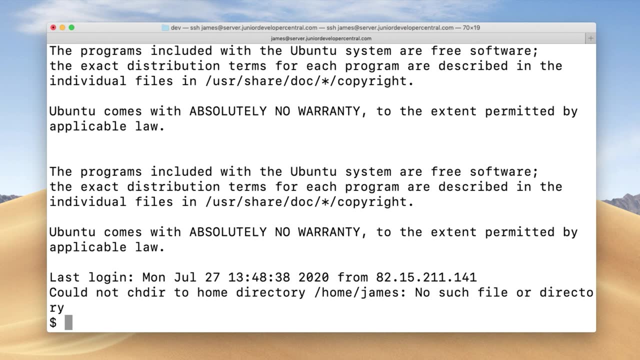 as the server host. Again, I'll enter the password for this user and once the SSH connection is established, I can then run commands. The other way to make an SSH connection is to use a key to prove you are authorized to access a server. This way, the server doesn't need to request a. 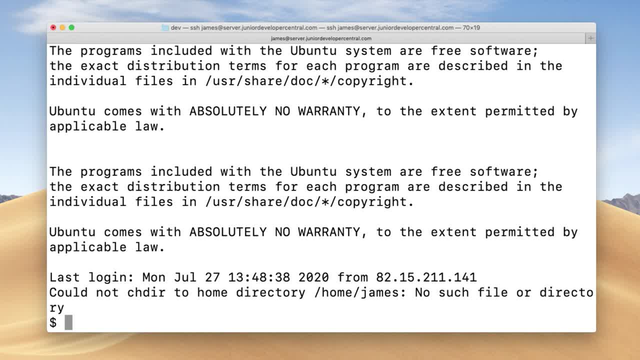 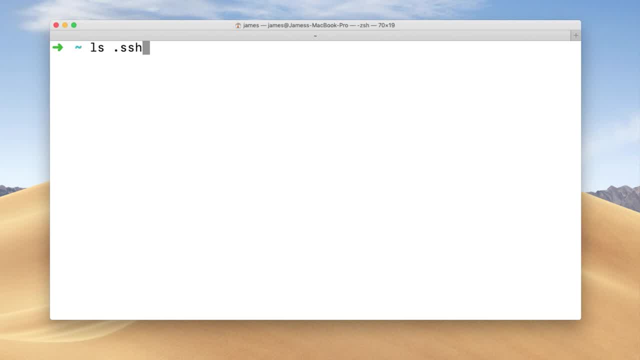 password when you connect, which is useful if you're setting up your SSH connection in a script or a continuous integration workflow. You can see your SSH keys in the hidden SSH folder of your local computer's home directory. The key consists of two parts: the public key and the 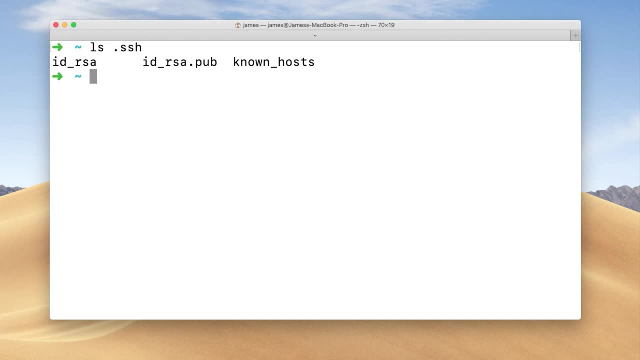 private key. The private key stays on your local computer and the public key can be provided to other resources, such as a remote server you want to connect to, to verify that the connection you create is from you. If you don't have any keys, you can create a new one with the. 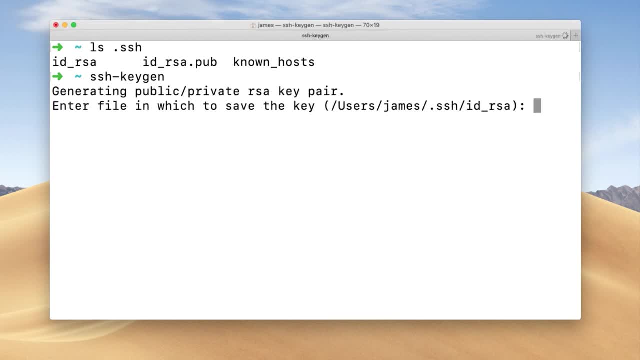 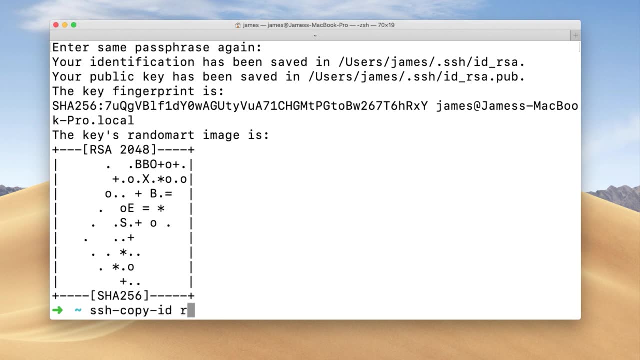 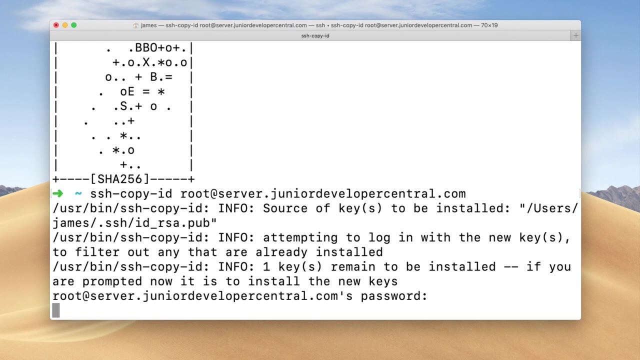 SSH keygen command specifying a name for the key and local password to use if required To provide your public key to a remote server. use the SSH copy ID command with a username and server, which will then copy your public key. Once the server has your public key, you can create an SSH. 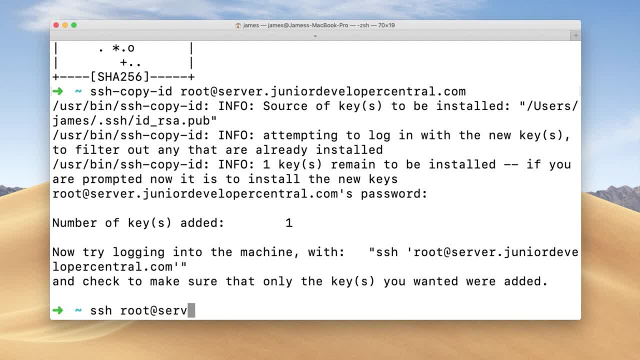 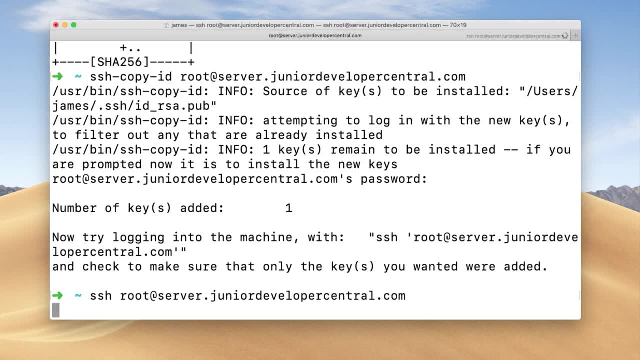 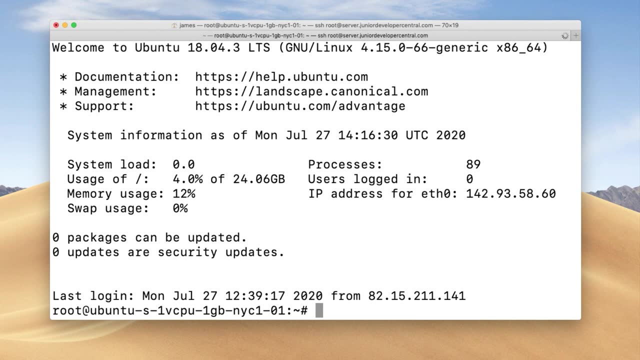 connection in the same way as before, but this time you won't be prompted to use the public key. Probably the most common other use of SSH for web developers is to copy your project files from your local computer to a remote server. There are several ways you can do this.